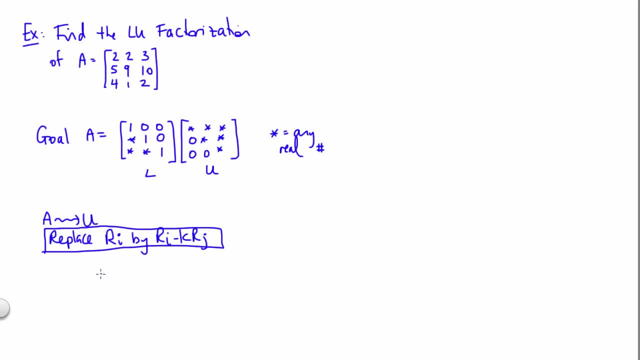 rephrase this. we're basically saying we're not allowed to swap rows, we're not allowed to multiply or divide rows through. we're only allowed to do this particular type of elementary row operation. So I'm going to recopy our matrix A and we can get started. What 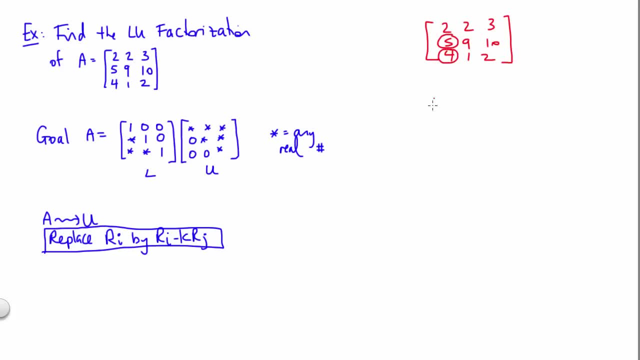 we'd like to do is get zeros in these two positions here. So we can first take row two and we can subtract off five halves of our pivot row, which will be row one. So we can check that if we go five minus five halves times two, that's going to 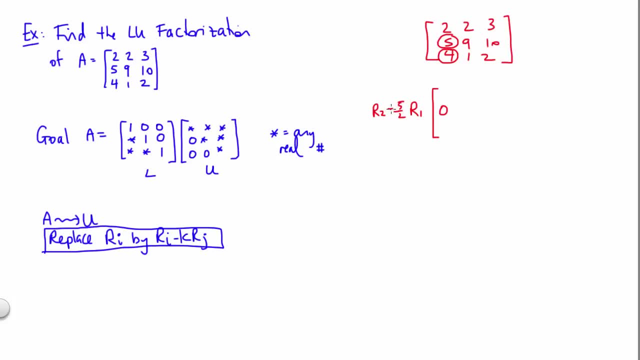 give us a zero in this position. So this is how we chose that multiple: that minus five halves there. To get a zero in the bottom left here, we'll have to do row three minus two times row one. Now, before we figure out all the entries in this, 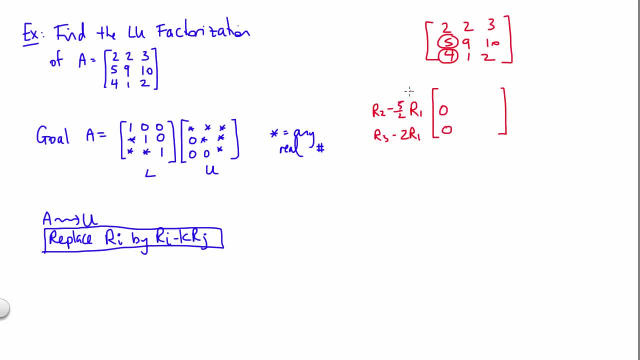 matrix. I want to point out that this multiple here that we're going to be using is going to be important when we write down our LU factorization. So beside the matrix, I like to record what the actual k value is And remember that the way that we defined our operation over here we said we're replacing row i by 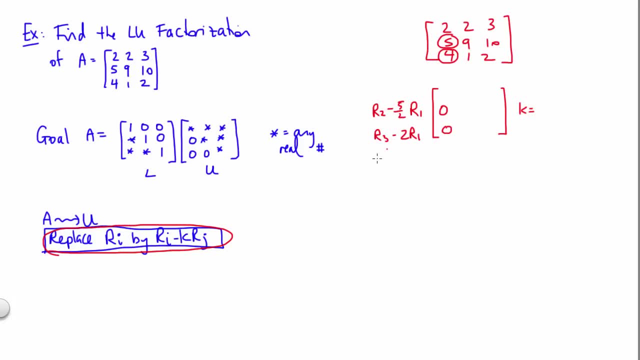 row i minus k, row j. So meaning if we've got a negative multiple here, k is going to be positive. k is actually positive five halves here. k is positive two here. So you can think of k as the multiple of the row that's being subtracted. 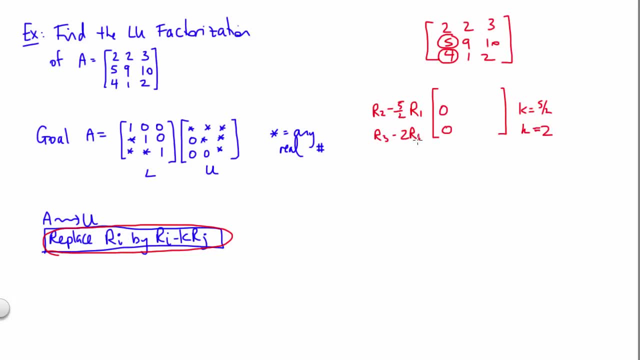 off. In other words, there's a sign change going on. Alright, so let's figure out the entries in our matrix. The top row stays the same: two, two, three. If we do row two minus five halves row one, we're going to have zero four, and if we want to do a, 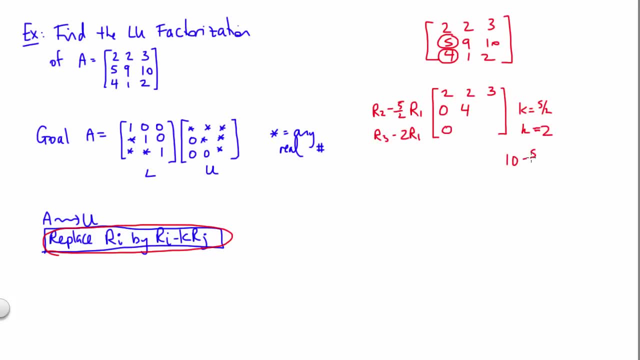 little calculation over on the side. here we'll have ten minus five halves times three, In other words twenty halves, minus fifteen halves, In other words five halves. Alright, so that's what's going in in this position here. I'm just going to keep this calculation out of the way. In the bottom row we'll have zero negative. 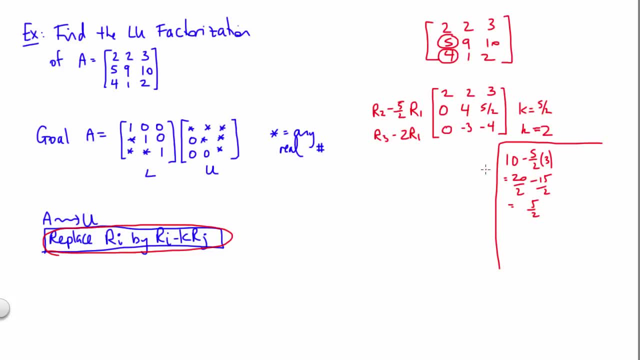 three and negative four. So that is our first step. all done, and we've remembered to record our k values again, watching for that sign change. So next step: we're going to try to get a zero in this position here. To eliminate this negative three, we're going to have to go row three plus three. 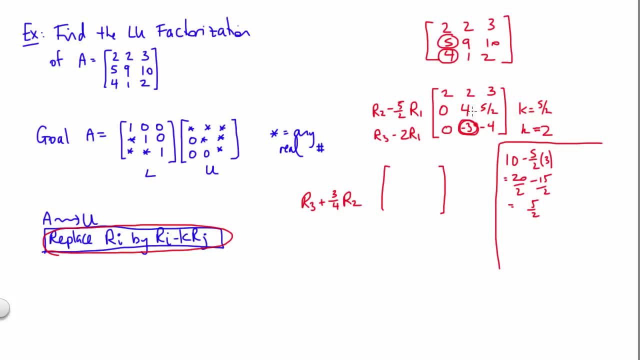 quarters row two. So we can just do a double check that, yeah, if we did negative three plus three quarters times four, that's going to give us a zero In that position. So that is the right multiple to use and if we want to record, 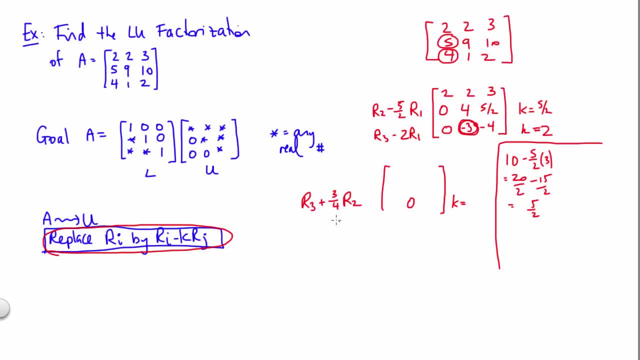 our k value here. remember, k is the multiple that we're subtracting off. In other words, there's a sign change going on here. k is negative three quarters. Alright, so we'll use this value. a little bit later on. Lets fill in our entries. 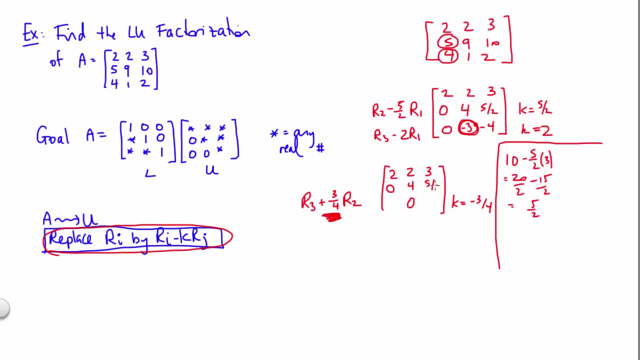 The top two rows are not changing and in the bottom row we've got zero, zero. and then we may need to do a little calculation here over on the side We've got negative 4 plus 3 quarters times 5 halves. So if we put everything over 8, we've got negative 32 over 8 plus 15 over 8 gives us. 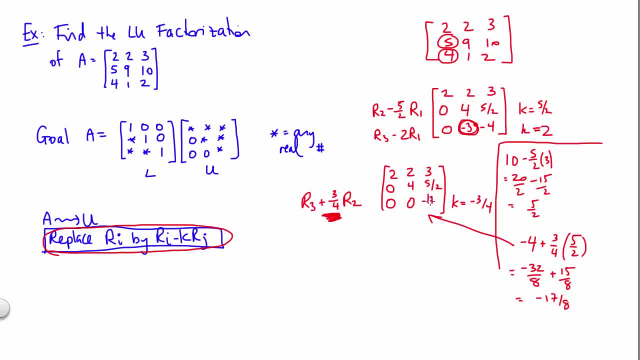 negative, 17 over 8.. And that's what's going to go in the bottom right-hand corner there. So at this point we have found an upper triangular matrix. This is the matrix U that we're going to be using in the LEU factorization, And to get the matrix L, we just need to know how. 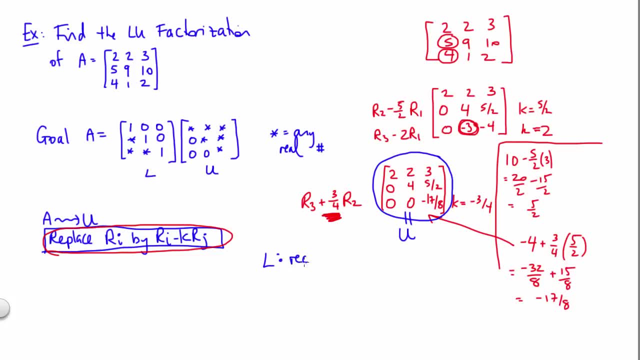 to build L. What L does is it records the k values in the appropriate positions. So let's take a look at that. So we've got a matrix U and we've got a matrix L and we've got a matrix L. 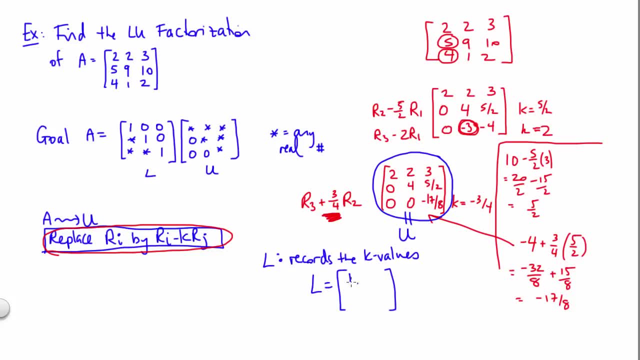 So let's take a look at that. So let's take a look at that. So let's take a look at that. So let's take a look at this matrix L. It's going to have 1s along the main diagonal, 0s above the.